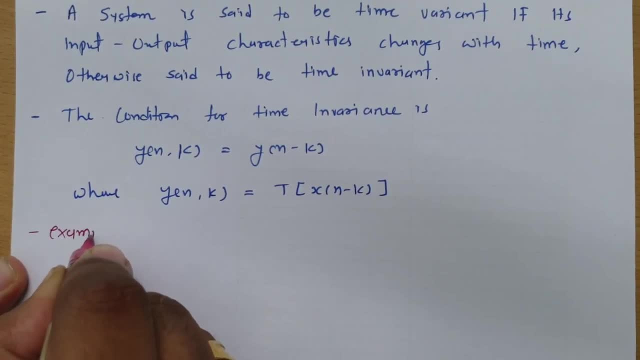 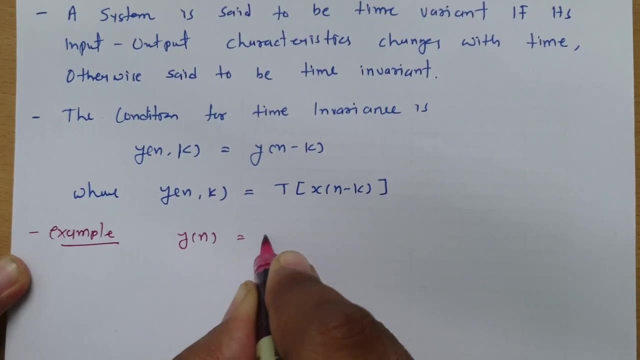 So let us have first example. Let us see: if question is y of n, that is given by x of n. So y of n k is equal to x of n minus k. For this product I will write n equal to x of n plus x of n minus 3.. 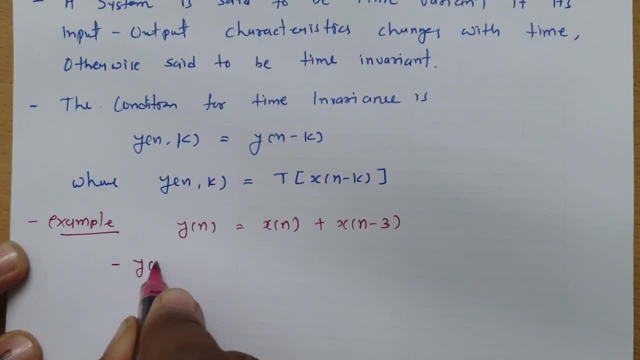 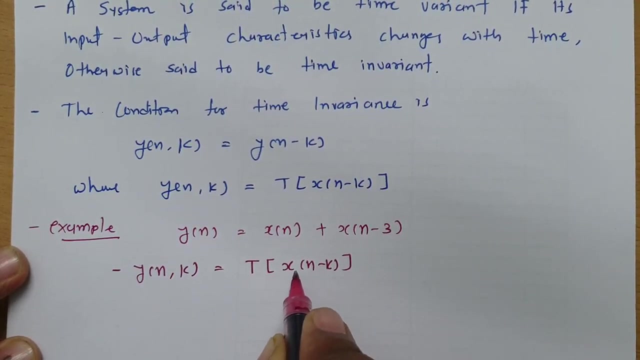 So in that case, if you calculate y of n k, So what is y of n? k? So that is transpose of x of n minus k. So here instead of x of n we need to replace it with x of n minus k. 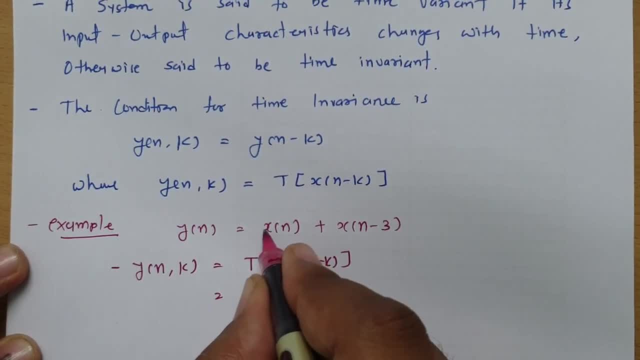 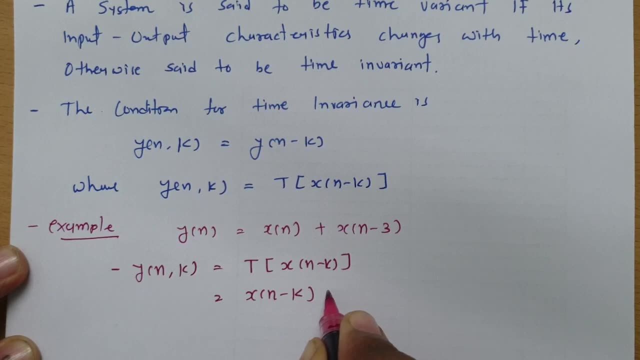 So over here, x of n, this is x of n minus 3.. So this is y of n minus k. This is x of n minus k. The values here are none. that will change is to X of n minus K. plus here, X of n minus 3 is there, so it. 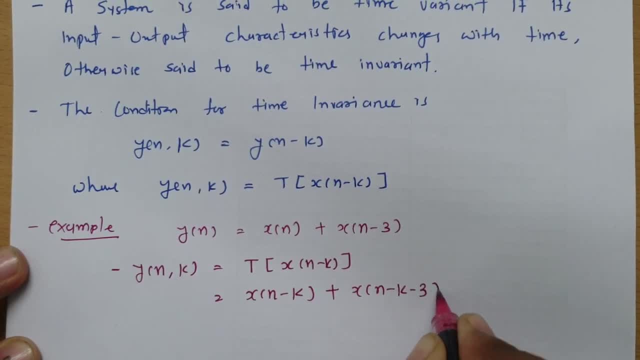 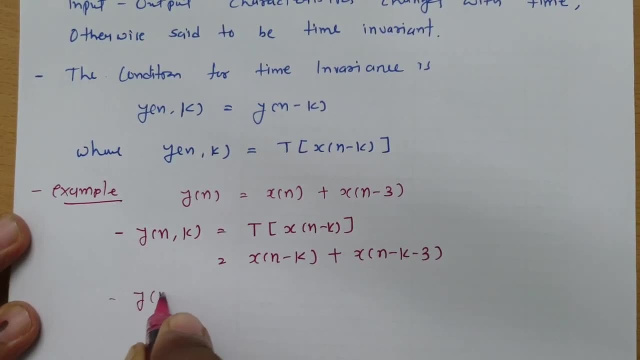 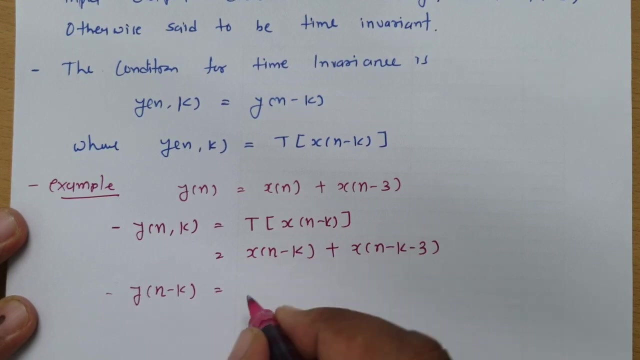 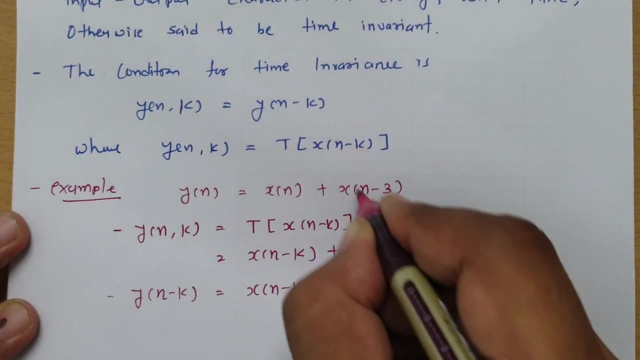 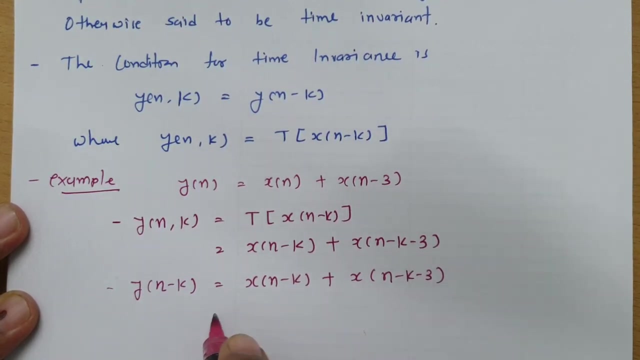 will change is to X of n minus K minus 3. now what is Y of n minus K? so in that we need to replace n with n minus K. so you will be finding that X of n is replaced by n minus K. so X of n minus 3. that will be now X of n minus K minus 3. so this is what actually. 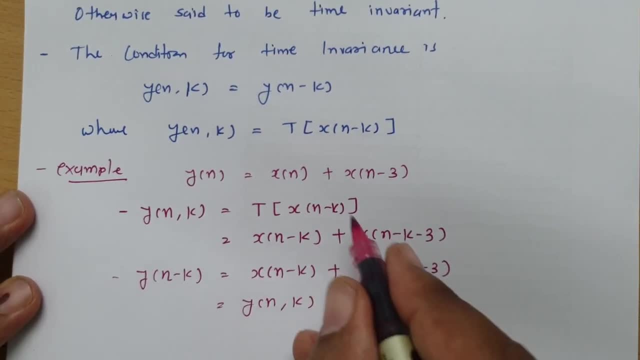 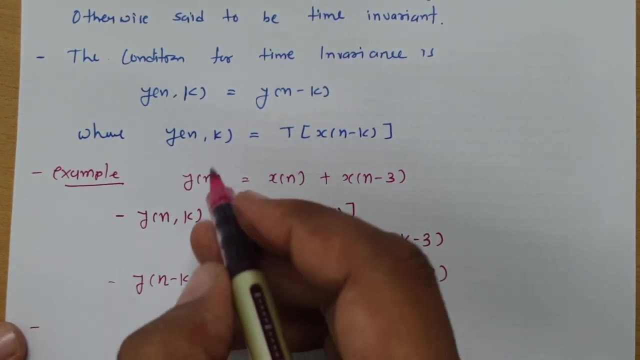 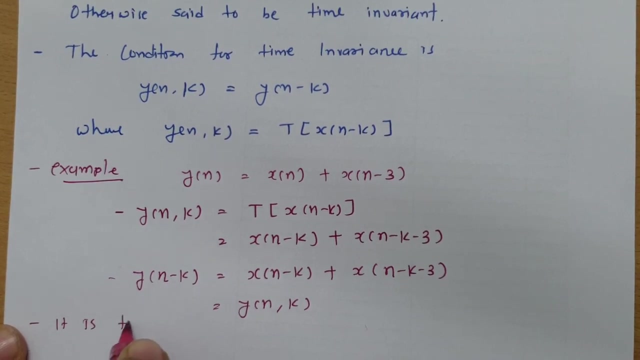 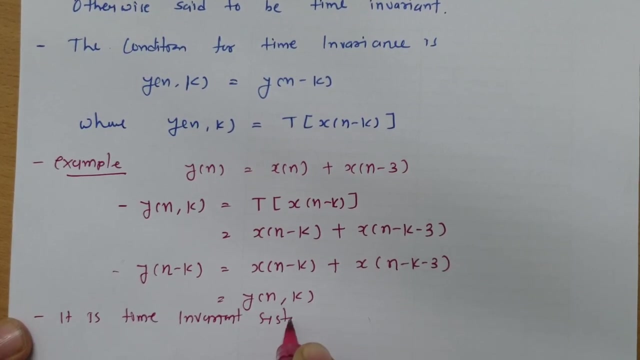 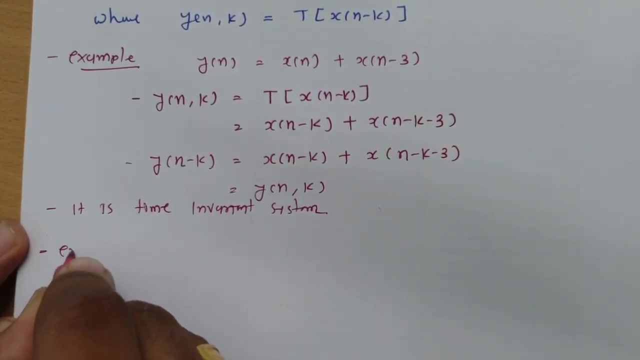 Y of n comma K. so we can say this given system is linear system. so this system follows the condition Y of n comma K is equals to Y of n minus K. so it is time. invariant system. now let us have few more examples so it will be more clear. so I am considering second example now. 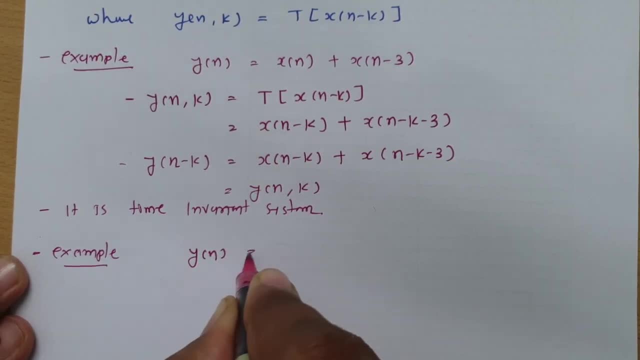 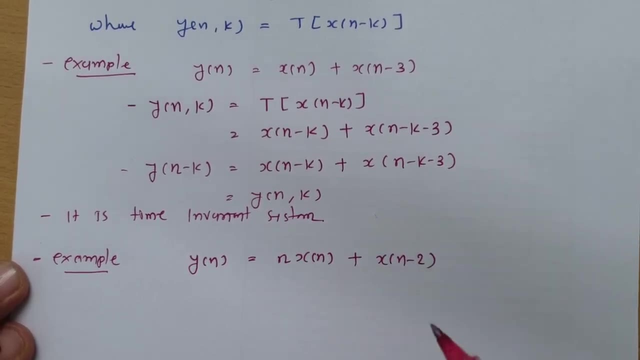 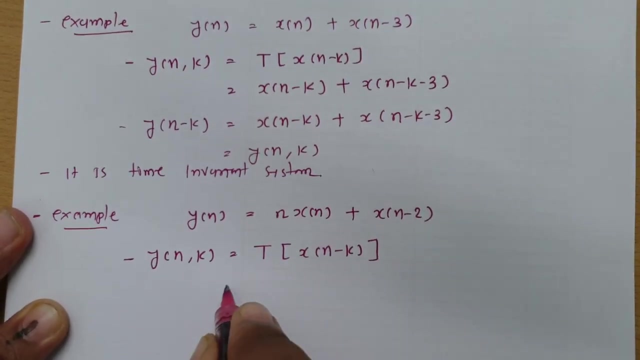 see if Y of n, that is given by n, into X of n plus X of n minus 2. so how to calculate Y of n comma K. so Y of n comma K means what it is a response: X of n minus K. so here you don't need to replace all n with 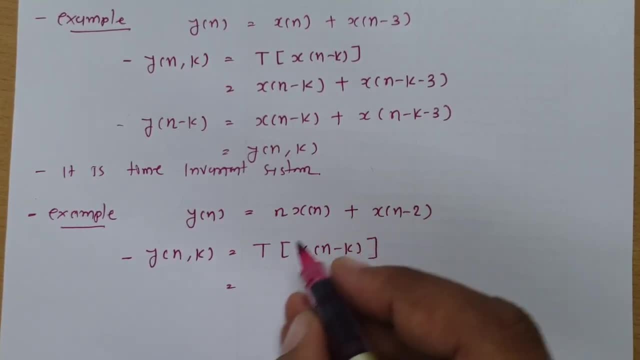 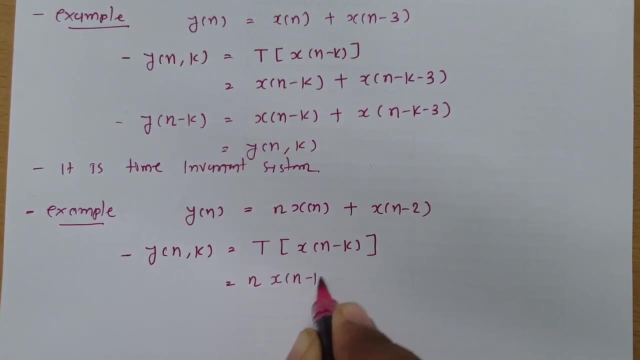 n minus K, you will have to replace only inputs. so here this n, that will be as it is, But X of n, now that will get replaced by x of n minus K plus X of n minus 2. so there you need to replace input with X of n minus K, so X of n minus k minus 2. so this is what. 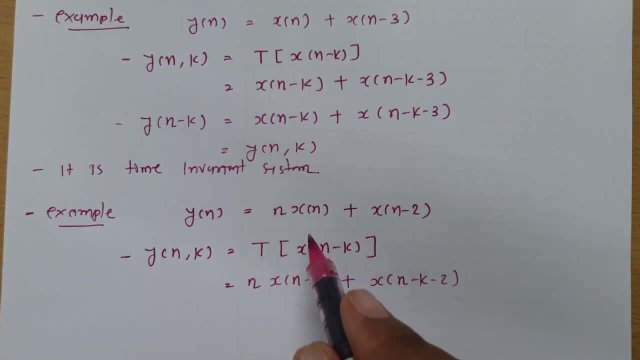 the difference. you don't need to replace all n with n minus k. you'll have to replace only inputs with n minus K. So Y of n comma k will replace will be Y of n comma 2. okay, will be this Now when you calculate y of n minus k. So in that case you will have to replace all. 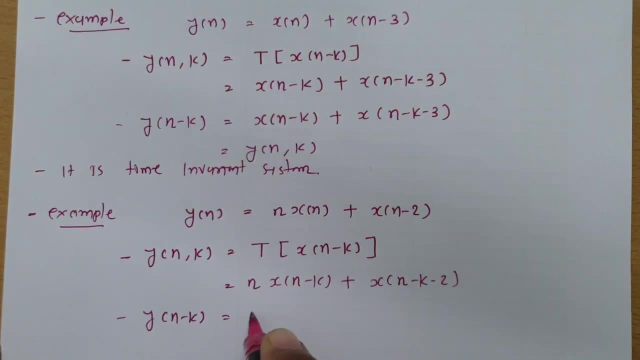 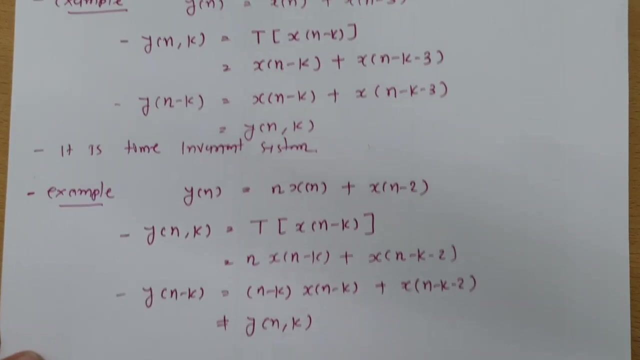 n with n minus k. So here n is there. So that will be now n minus k and x of n minus k plus x of n minus k minus 2.. So this is not equals to y of n comma k. So we can say here characteristic. 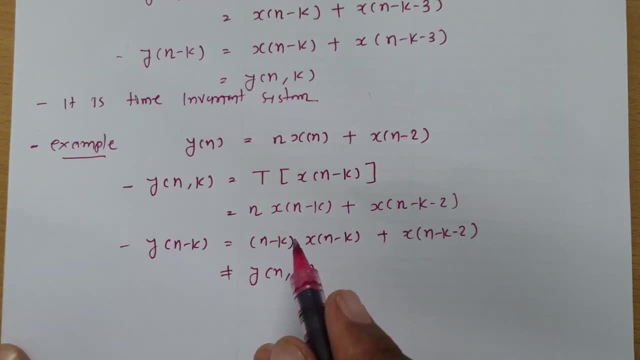 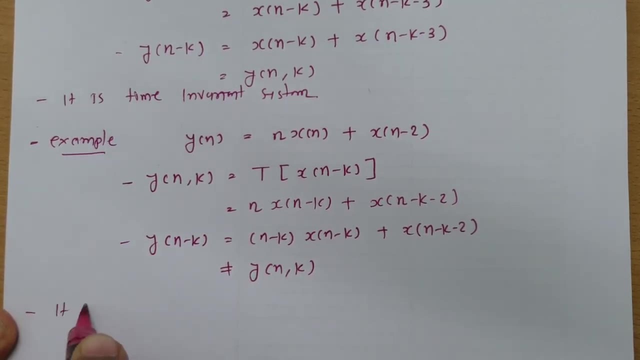 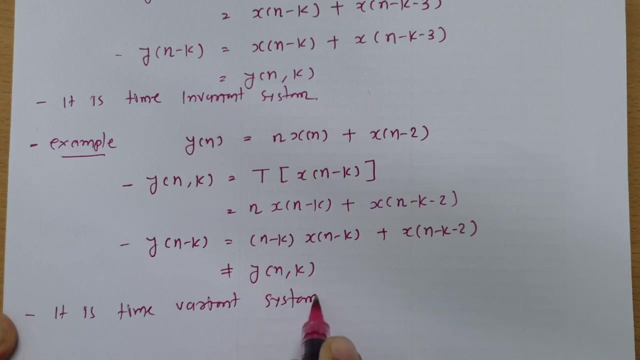 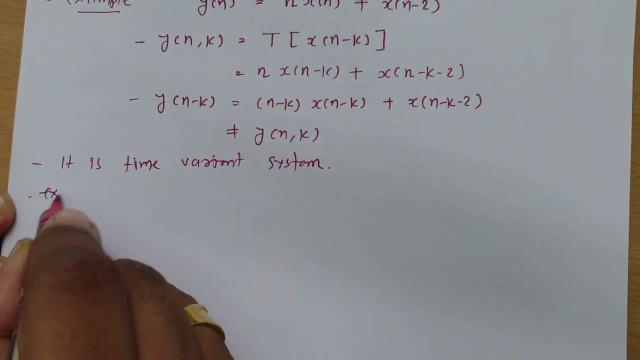 of system is changing with respect to time And as characteristic of system is changing with respect to time, one can say: it is what? time variant system? So this is time variant system. Let us have one more example so it will be more clear. So I am considering third. 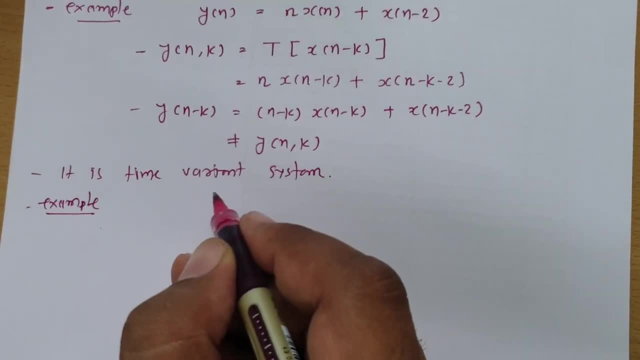 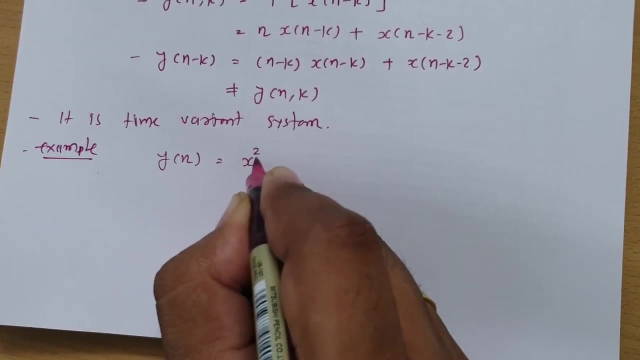 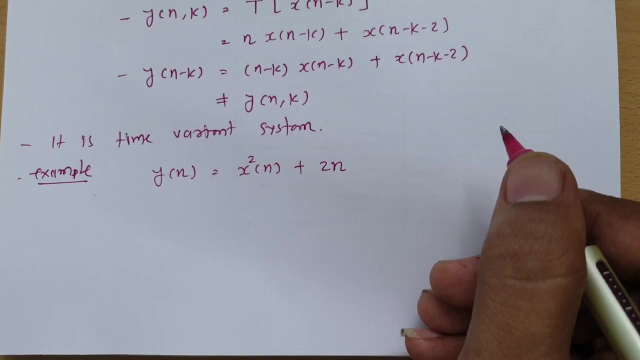 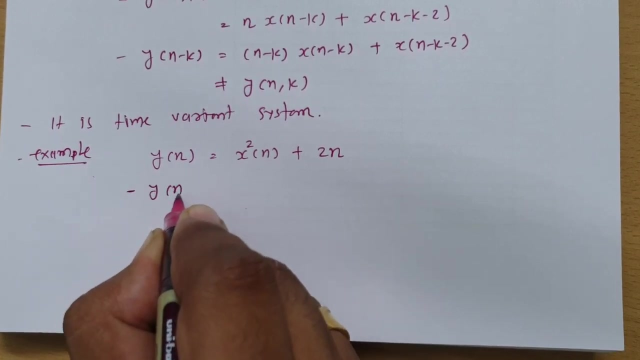 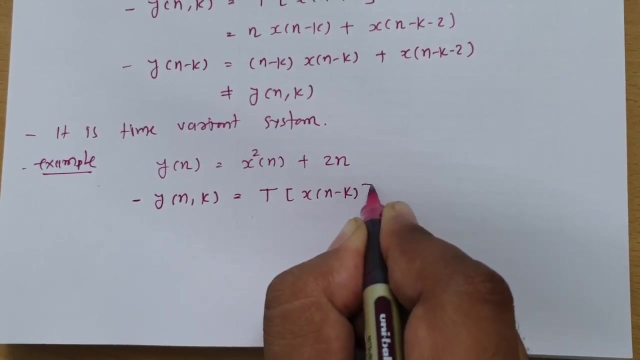 example. Now see if you have y of n, that is x square n plus 2 n. So now we are going to identify whether this is time variant or not. So if I calculate y of n comma k, So that is actually transpose of x of n minus k. So we need to replace x of n. 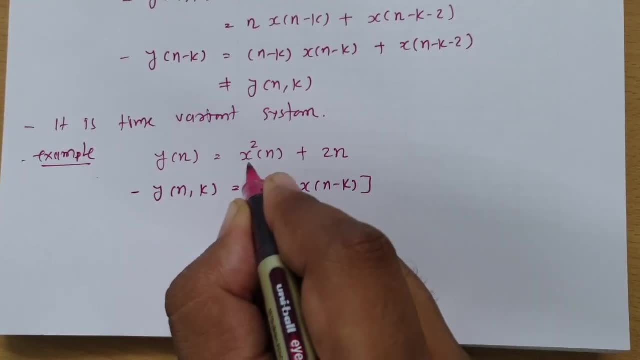 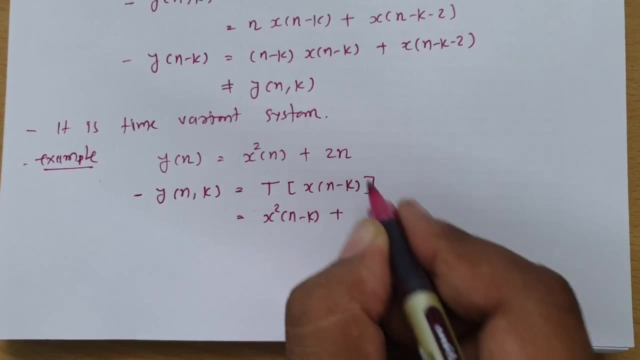 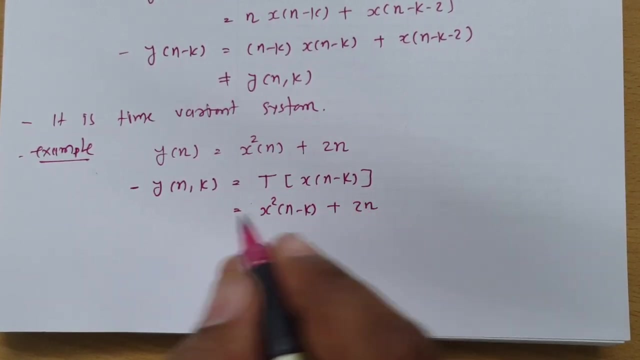 With x of n minus k. So here x of n, that is given, So x square of n minus k. But you cannot replace this 2 n. It will be 2 n as it is. So x of n comma k is this, And if you calculate,